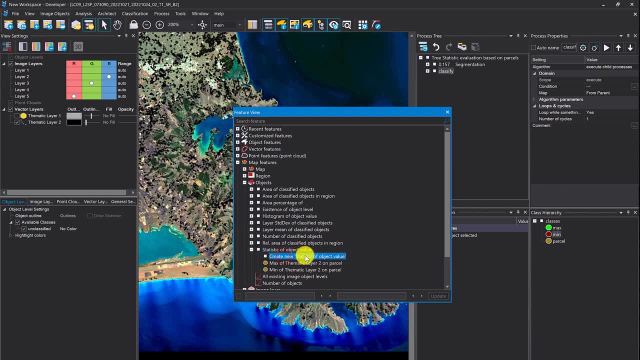 statistic of object value. and if you double click this statistic of object value, this create new, you're gonna get these options here. So what can you define here? Class? that's one parameter. I have different class, so you select the class you want to compute statistics for here and then with. 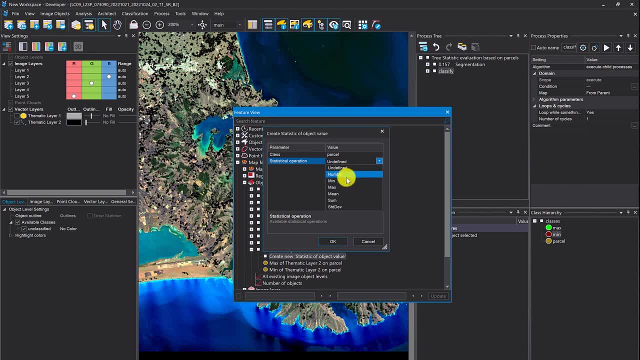 different statistical operations, undefined number. min, max mean some standard deviation and you, for example, could compute the mean value and then you can select a feature from the feature list and then what it will do: it will create or compute this statistical operation to the mean of the feature that you've selected here, only for the classes selected here. 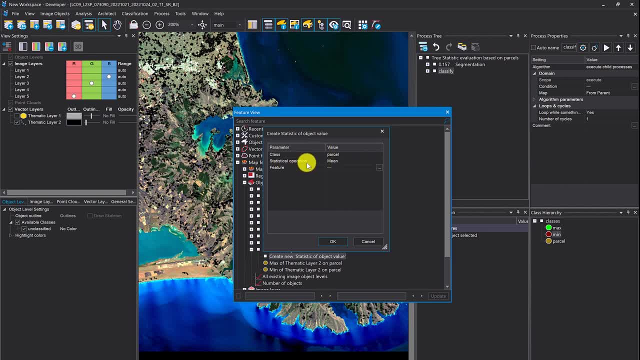 So for all parser classes, it computes the mean of this feature, so it won't include the other classes or unclassified right. So you will get one value which represents the mean of all those objects classified as parcel, in this case of a certain feature. And yeah, I'm quickly gonna show you how I'm gonna put. 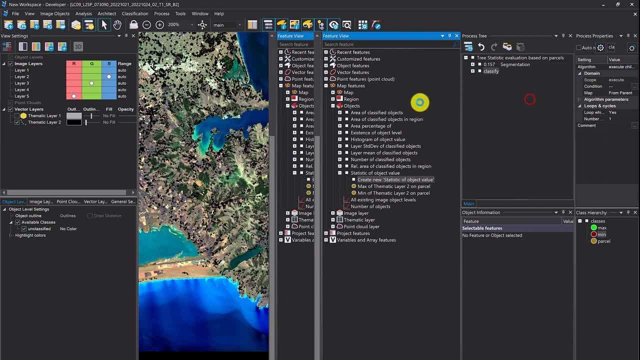 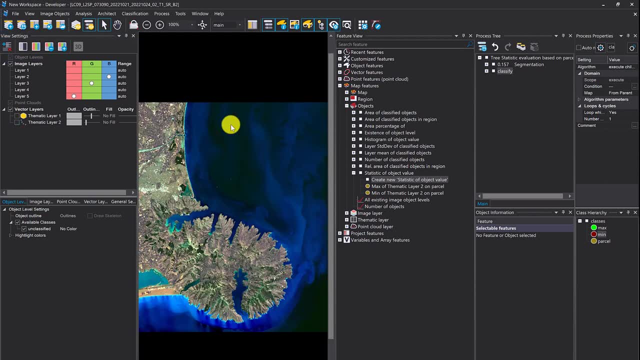 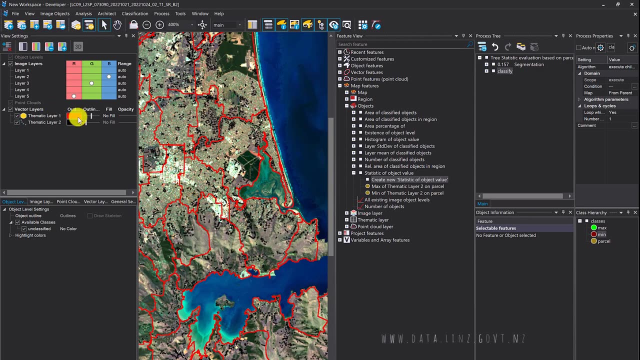 it here, how you could use that in a project. So a small use case here. What you see here in the view is image, and I do have one thematic layer representing my parcels and another one with points. Those are single trees. And now I'm actually interested in statistics of the 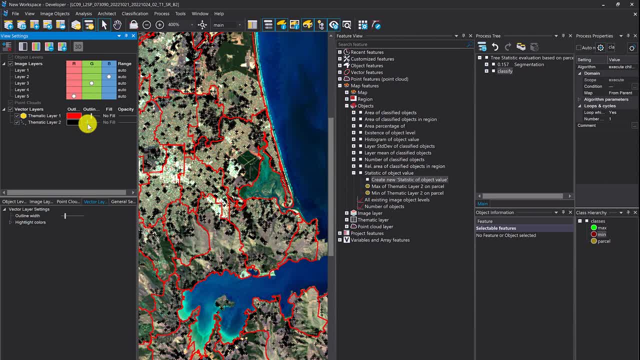 parcels regarding the trees. So what is the parcel with the highest number of trees? Which is the parcel with the lowest number of trees? And what's the lowest number of trees? What is the mean? So statistics about the parcels in my project. So what I first do here is I: 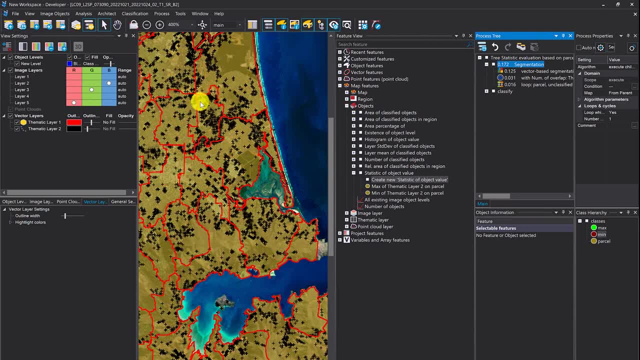 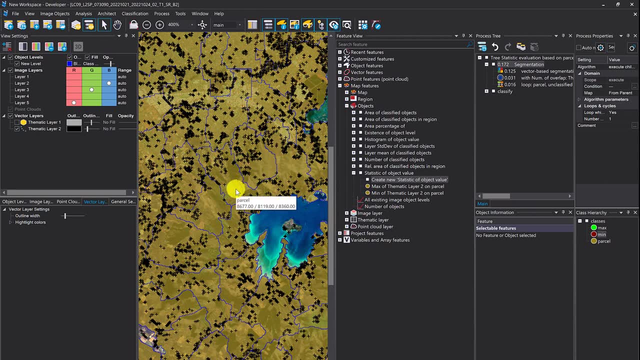 do a segmentation and classify those parcels. So I have image objects that are representing the parcels and I classified them here into this yellow goldish color And now we can have a look at this statistic of object value. Let's assume you want to know the total number of trees within all of your 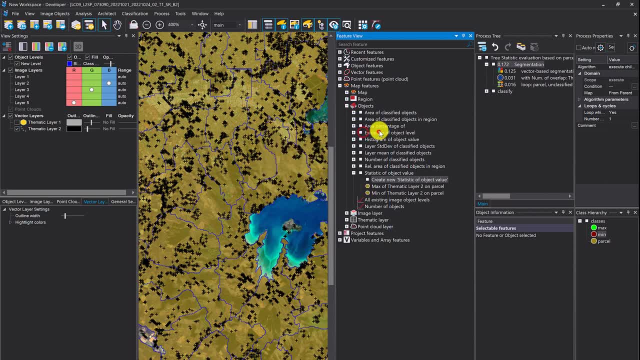 parcel objects. What you have to do is go into feature view and the map features Objects, statistics of object values. Double click this, create new. Then you have to select the class- In our case it's parcel. Then we want to have the sum. 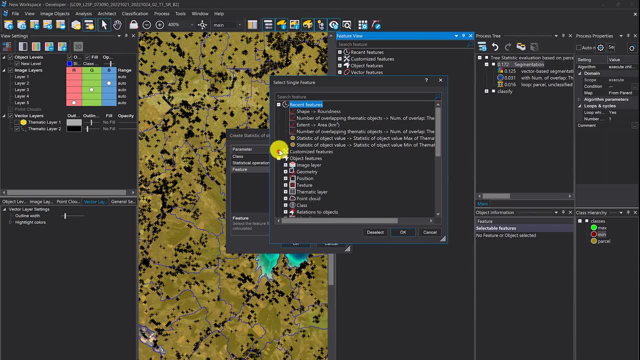 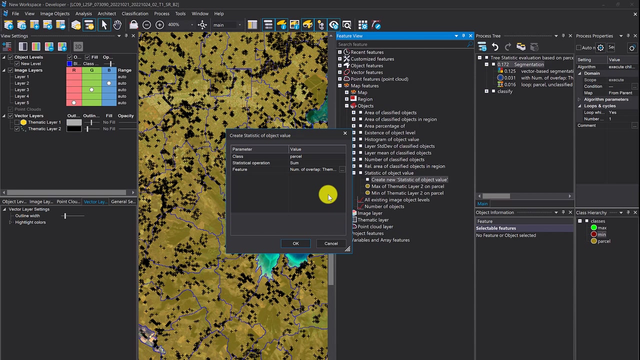 And the feature is number of those points within one object And this can be found here under object features, thematic layer Overlap And I think I already created the number of overlapping thematic objects. This feature gives you the number of overlapping thematic objects. 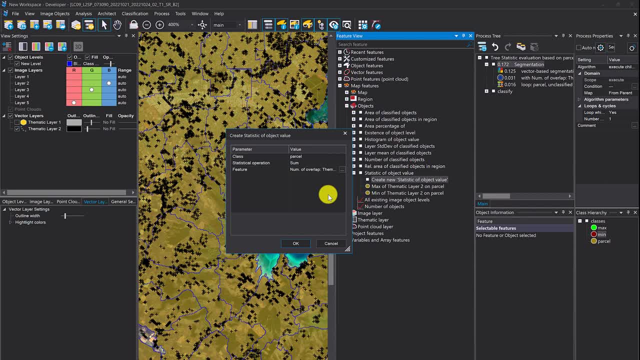 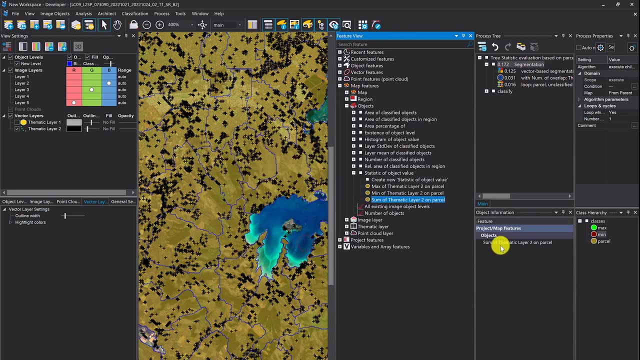 per object. So it simply counts how many trees, in this case, are within one object. And this statistic of object value now sums up all of those numbers for each object that's classified as parcel And gives me that value. Image, object information. Let's put it here: 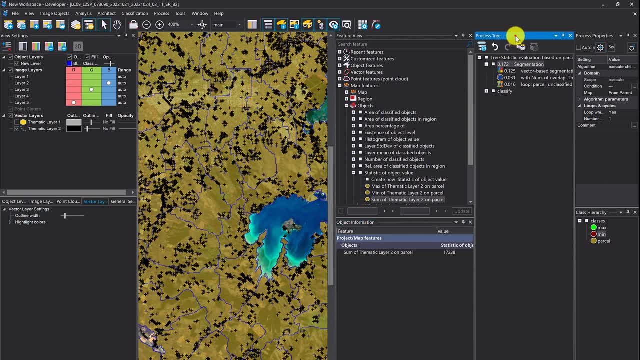 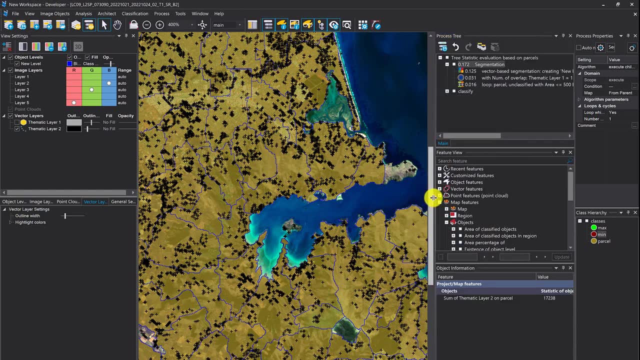 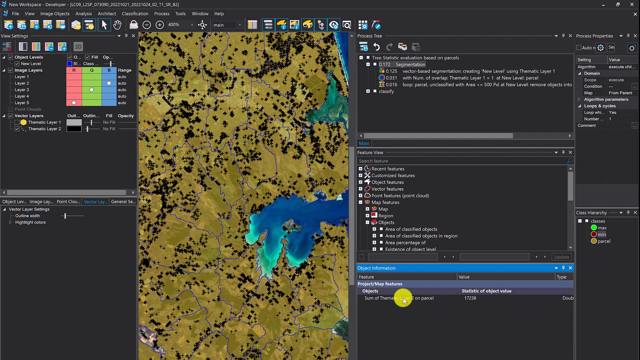 Okay, I have to put it here. All right, That's good, And let's resize the window. So you see here sum of thematic layer two on parcels. Thematic layer two are the trees on parcels, So only parcels. In total we have 17,238 trees. Now let's say: 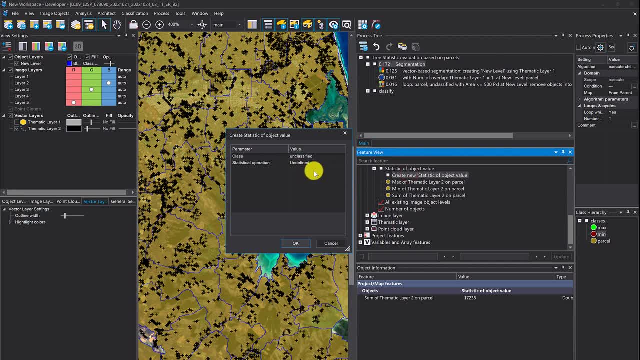 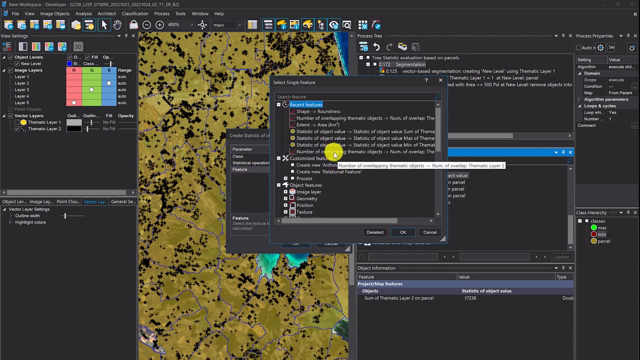 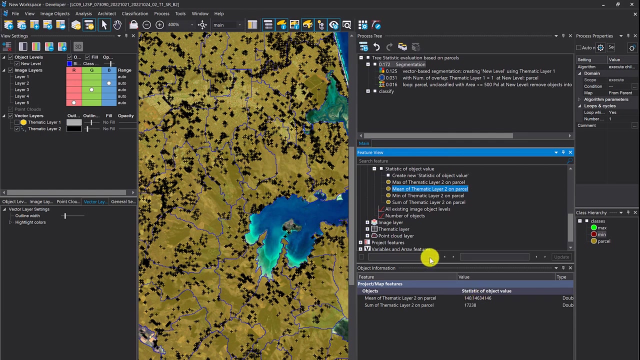 we are interested in the mean value. All right, Same procedure. We select parcel here. in this create statistic of object value. We now select different statistical operation And the feature is the same. It's number of overlapping thematic objects. Number of overlap thematic layer two. Okay, The mean is 140.. Now one more parcel. 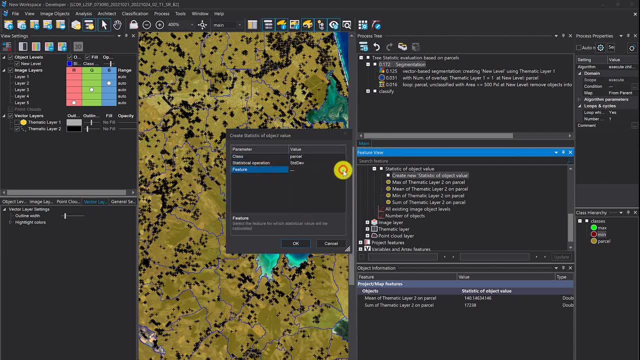 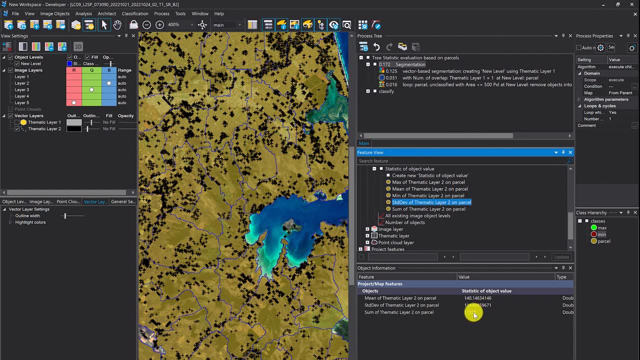 Let's go for standard deviation, So we have a better understanding of the distribution. And let's go for standard deviation. Standard deviation is 114.. Okay, Interesting, I already created the min and max, So I'm going to display it here as well. Map features- All right. 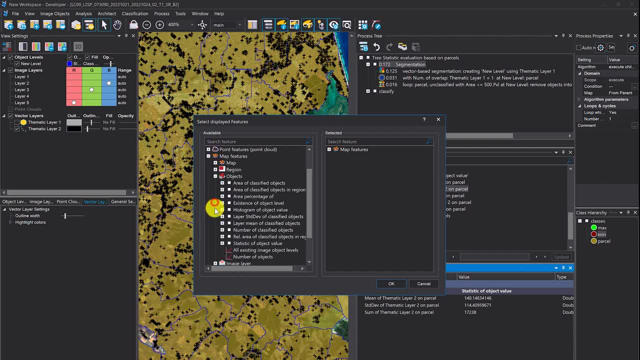 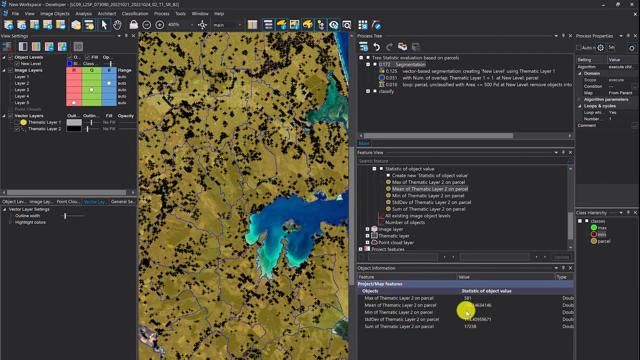 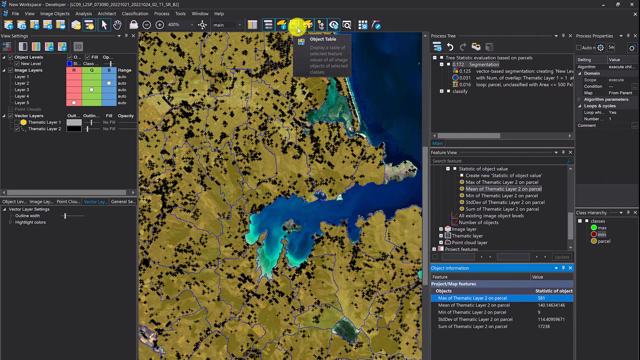 objects statistics. here we go, those two. i want to have them as well in here, and you see, the minimum is nine and the maximum is 581. now i want to classify those objects right. um. one tool that i think a lot of users are not using is the object table. this is so cool because you can 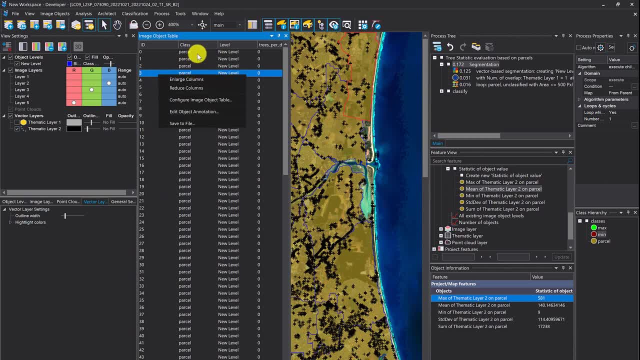 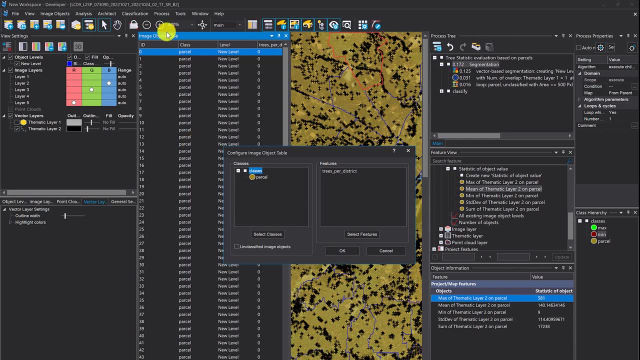 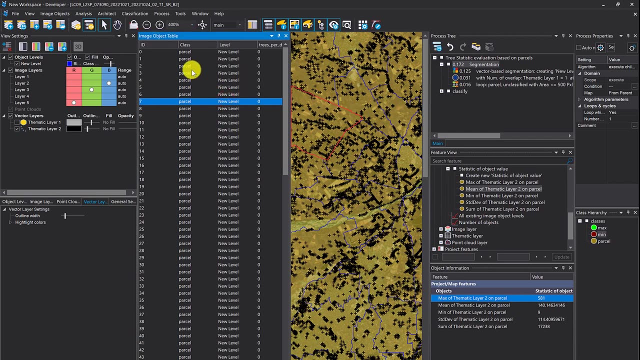 actually plot or display in a table format your objects and features. so what you can do is you can select the class. i only want to display parcels and the feature, okay, and that's going to display all of my objects here, and i need to change the feature. 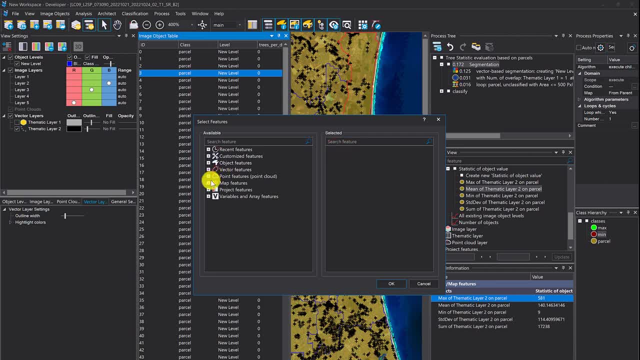 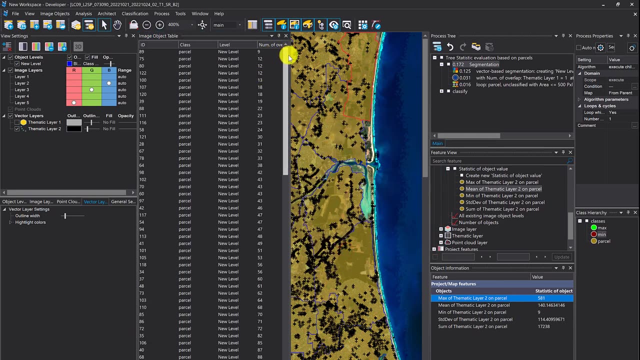 so i want to have the number um, so, um, um, how is it called overlap, number of overlapping? so i want to have the number of trees per parcel. and the cool thing about this image object table is that you can sort- actually right- and you can click on those entries and the object is going to be highlighted and centered in. 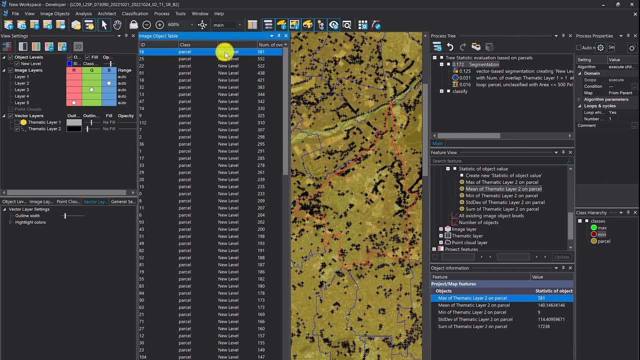 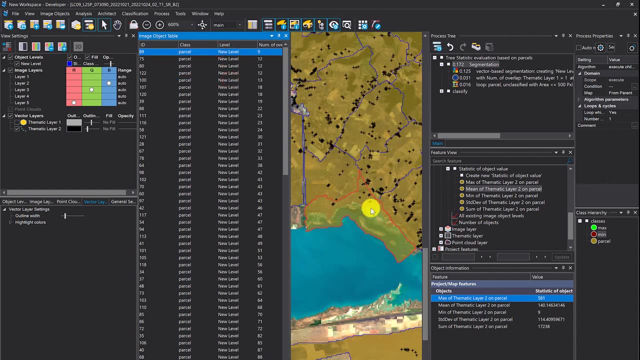 the view. so let's see if this is consistent. so 581 is the highest number of trees and the highest number we get here, and that's also the output of the feature that we've computed. what's the lowest number? it's down here, nine. it's this object, here, nine trees um, and that's also. 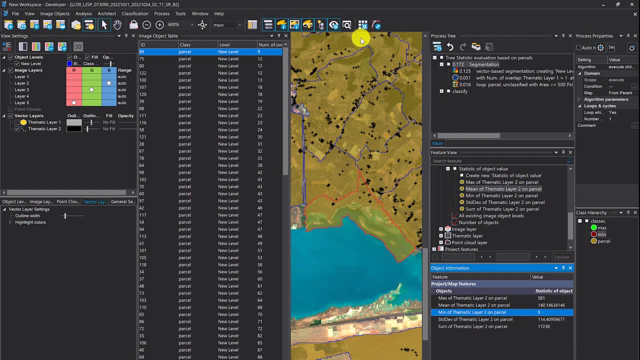 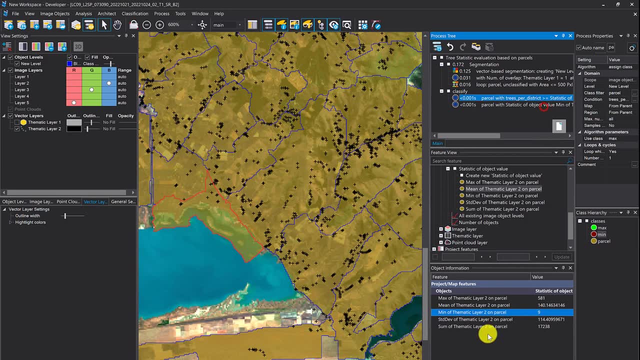 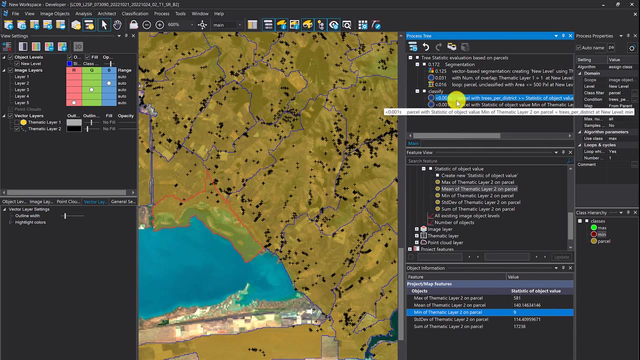 consistent here with the feature. if you now want to classify it, um you well, what i'm doing here is i'm using the assign class and i simply say: all right, if the number of tree objects equal the maximum number, then i classify you into the class max, and if it's the other way around, if